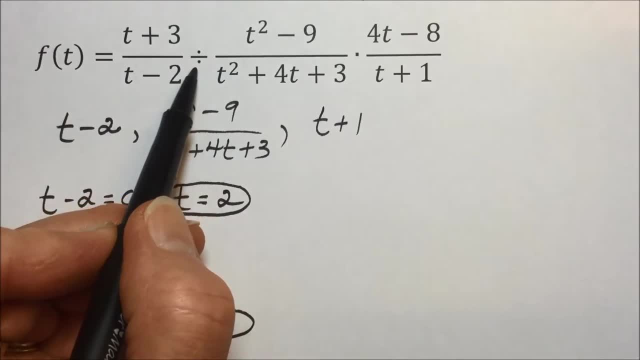 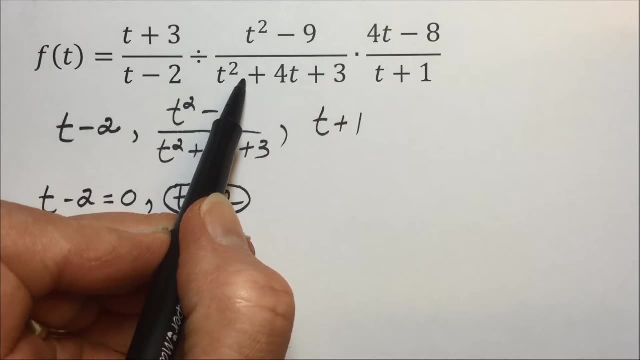 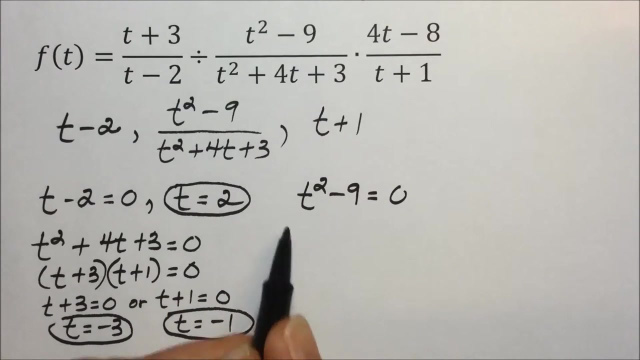 to muster 2 times the numerator and a 1 plus 2.. So the numerator has a 2 times the denominator, is each time 4 numbers are divided out in the denominator And this number here can be defined as the divisor number, because the denominator is 6 times 1. dressed under: 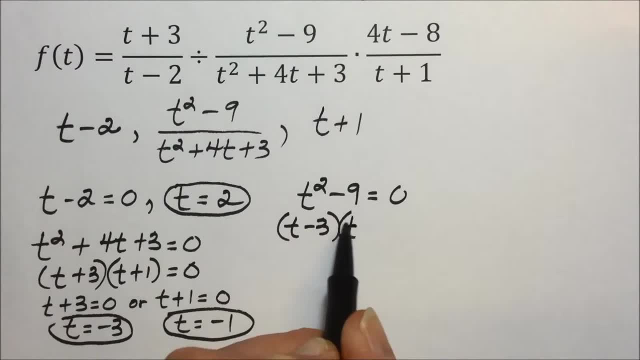 positive in and also treats the denominator as a divisor. And if you're caring about decreasing the denominator, the denominatoridiom is going to also be divided by its rational expression in The product of two things: equals 0 means t minus 3 equals 0, or t plus 3 equals 0. 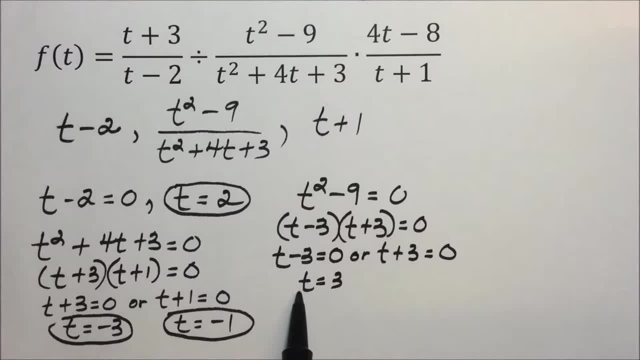 Adding a 3 to both sides, we have a restriction of t equals 3.. And subtracting a 3 from each side, we get a negative 3.. Well, we already had our negative 3, but we now add a t equal 3 for our restriction. 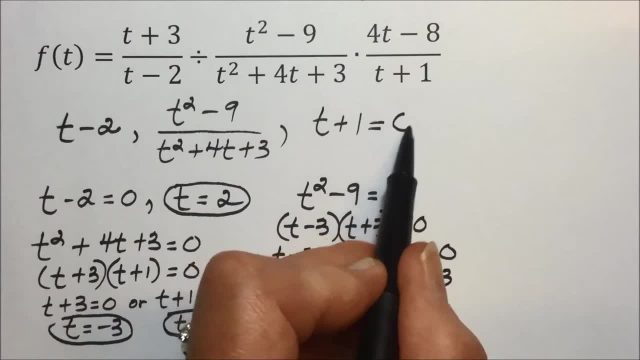 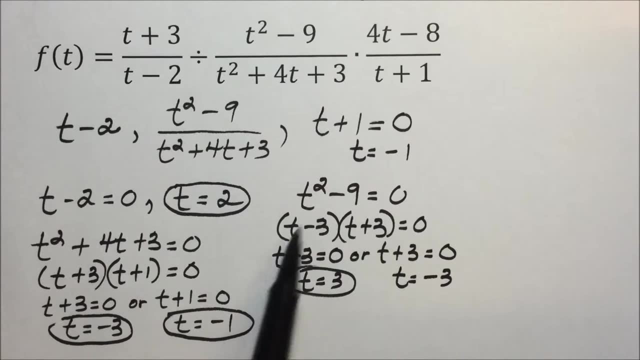 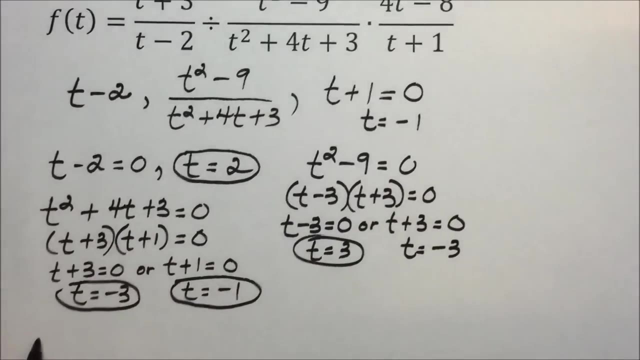 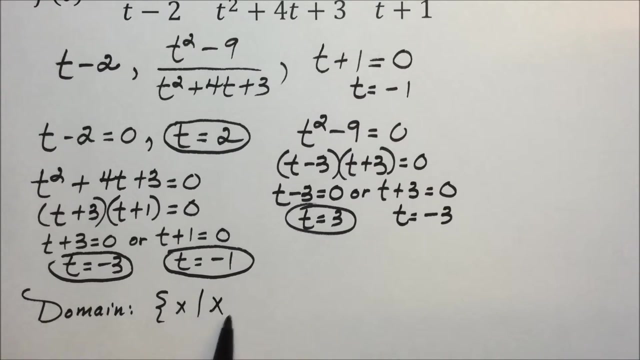 And our last one is our denominator here. When will it equal 0?? Something we want to avoid. When we subtract a 1,, we end up with t is equal to a negative 1,, which was also part of our list. So our domain will be x, such that x is an element of all real numbers. 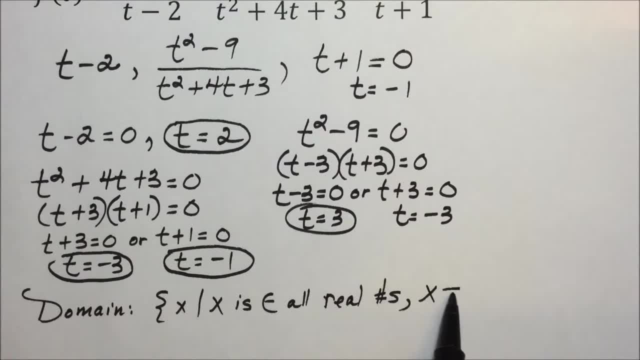 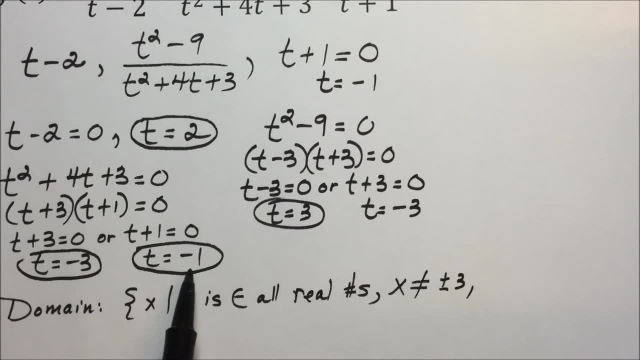 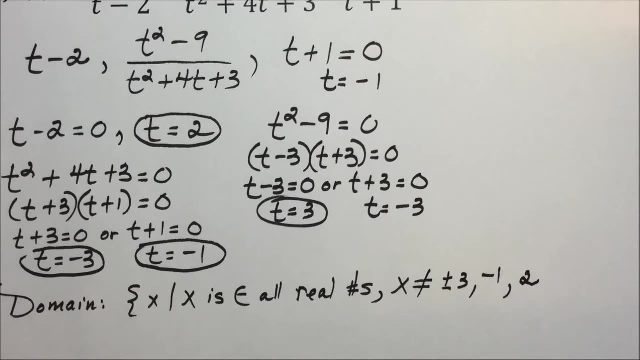 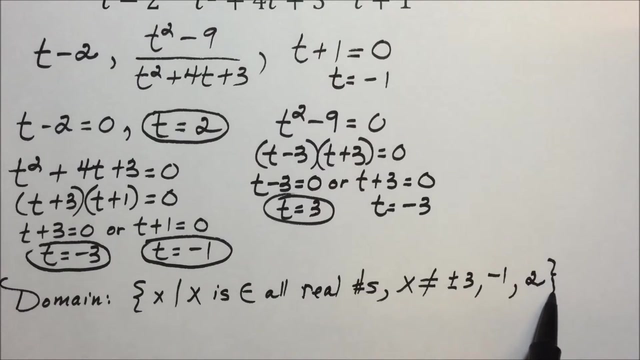 Except x, cannot be a positive and negative 3. It cannot be a 1, negative, 1. And it also cannot be a 2.. Those are the values that are part of our restriction, so that we don't run into a division by zero error. 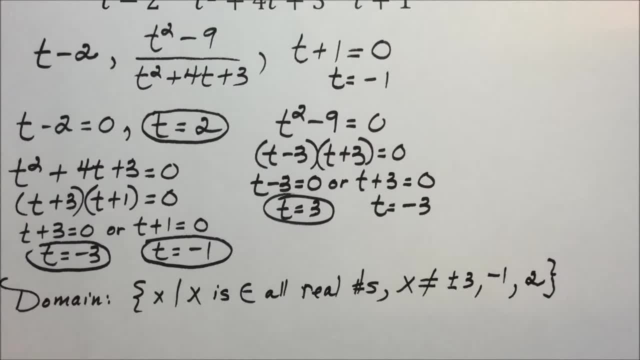 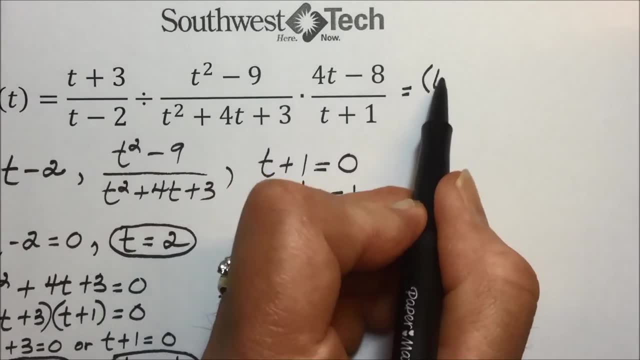 So what we're going to do is we're going to look at our function and simplify it. So nothing as far as factoring our first rational expression. 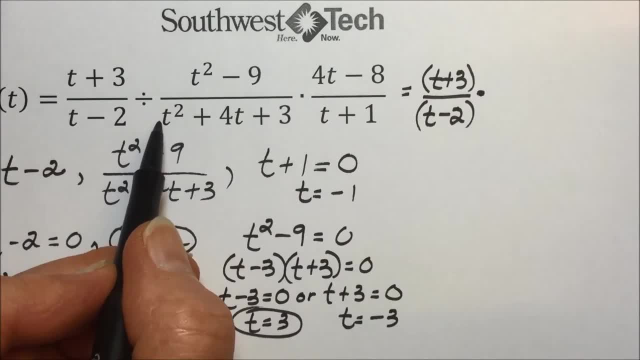 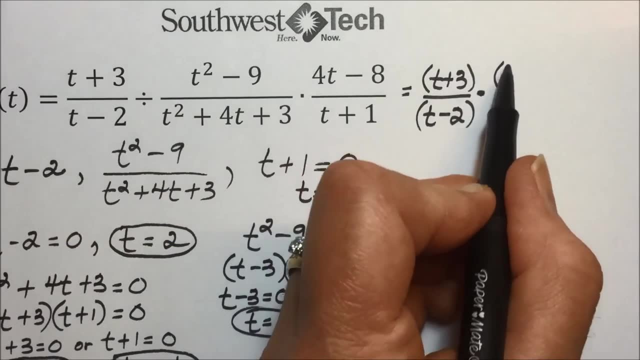 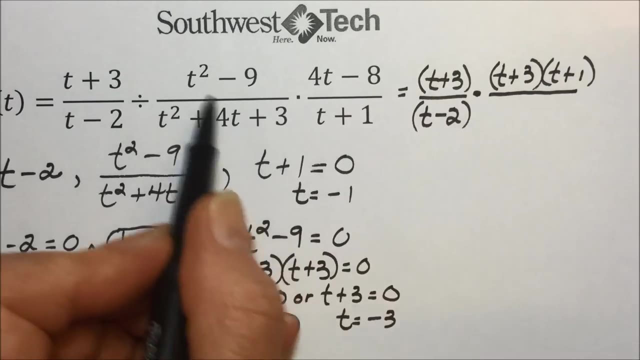 Division means we invert and multiply, so this fraction will switch places. The t squared plus 4t plus 3 will go to the numerator, which factors into a t plus 3, and a t plus 1.. The denominator is a difference of squares.